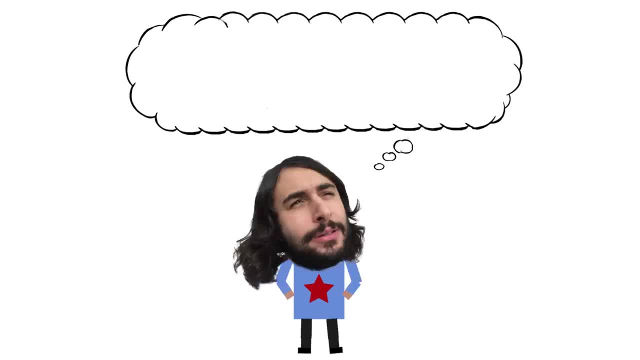 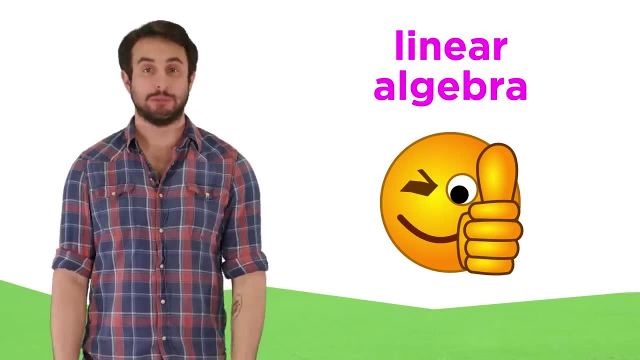 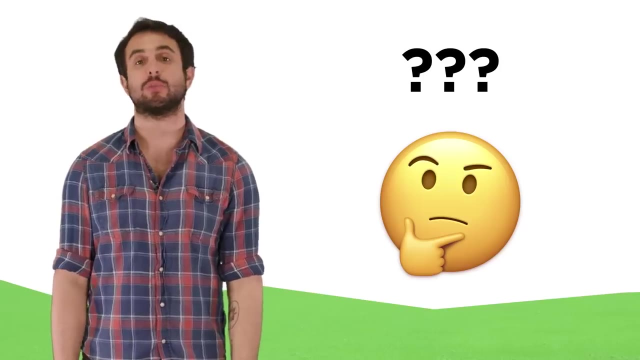 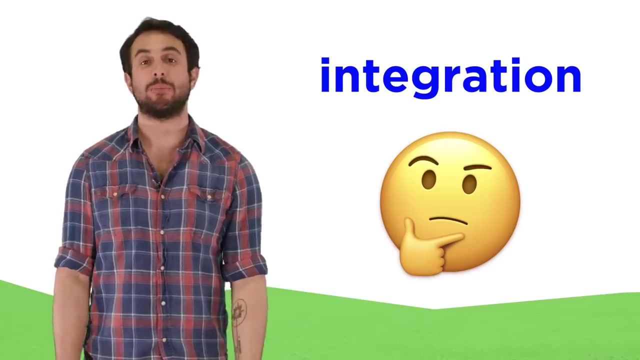 Professor Dave, again let's revisit integration. We've pretty much wrapped up linear algebra, but before diving into more advanced topics, let's use a few tutorials to go over some things we haven't covered yet. First off, let's go back to integration and see what happens when we find double or. 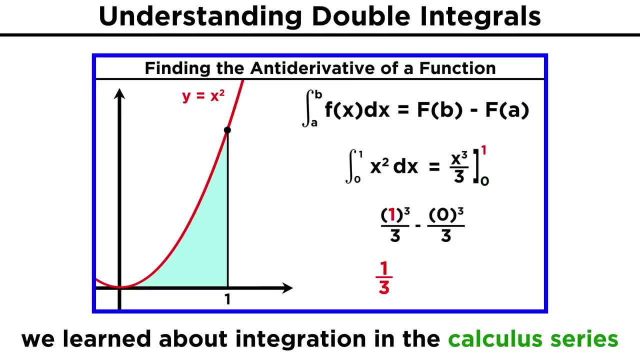 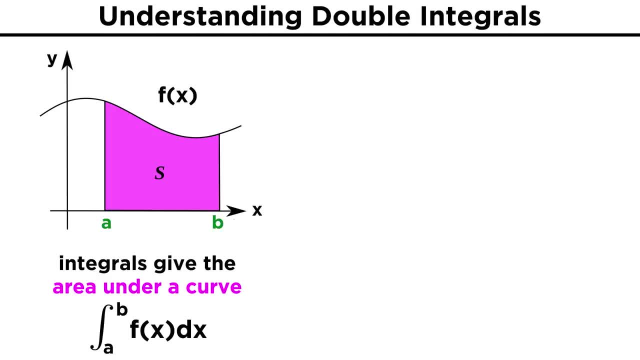 triple integrals. We spent more than a dozen tutorials going over integration in depth in the calculus series and we learned that it is a useful tool to find the area beneath a curve given by some function f. Now let's add a dimension. We can think of double integrals as giving the volume beneath a surface given by the. 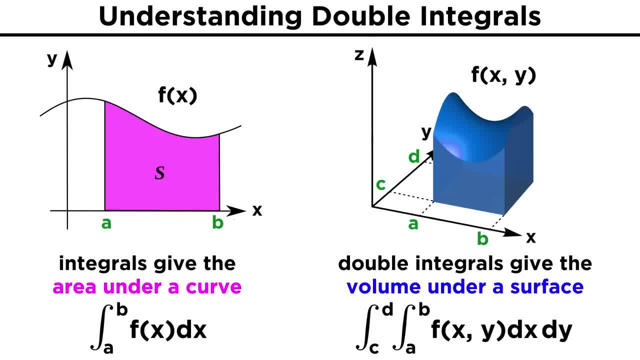 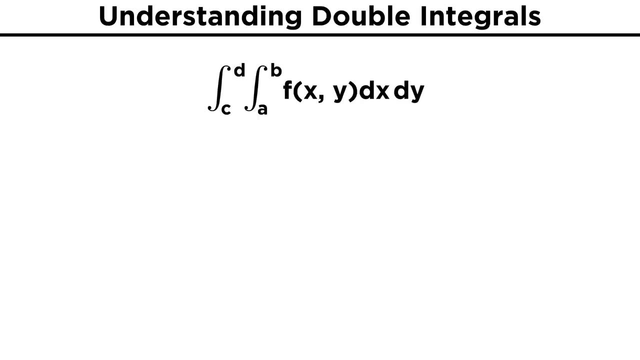 function f. We are now integrating over two variables, x and y. So for each variable we have an integration sign and to indicate the variables involved we have dx and dy. Performing multiple integrations is not all that daunting on the surface, it's simply. 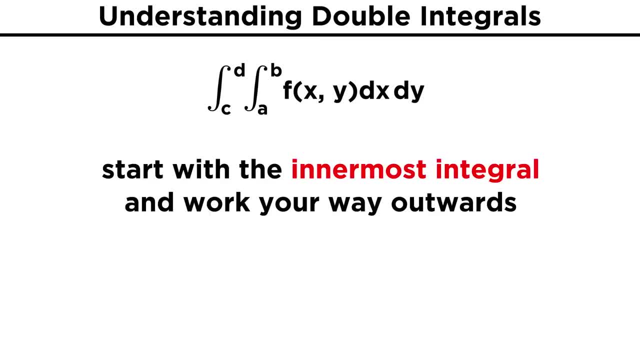 a matter of doing the innermost integral first and then moving outwards. We can use parentheses to more concretely illustrate this: doing the dx integral inside first, while treating y as a constant, Then integrating the result over y. We can use parentheses to more concretely illustrate this: doing the dx integral inside first, while treating y as a constant. 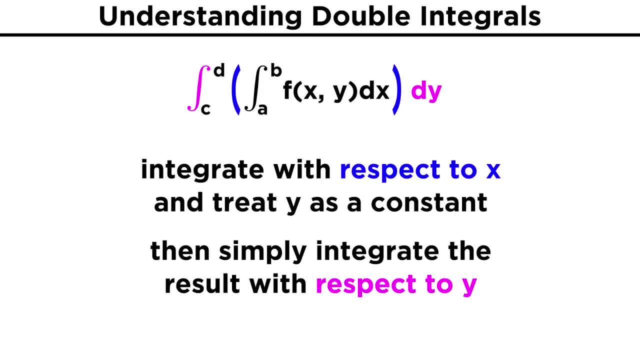 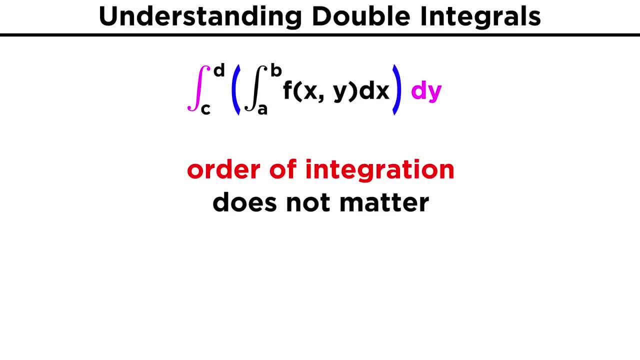 Then integrating the result over y. Just the same as we would for any variable. We can use the same as we would for any variable. The order in which we do the integrations does not matter, as long as we keep track of which variable has which bounds. 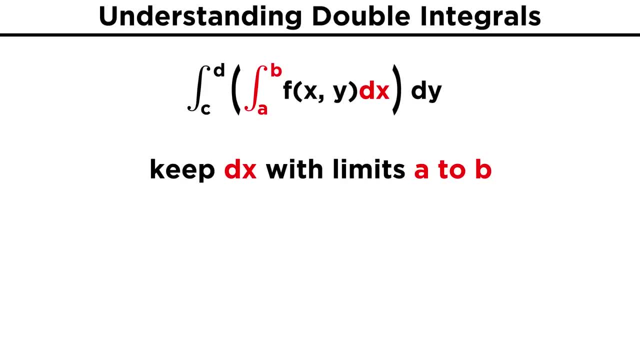 In this example we see that dx is associated with the x-integrant, which runs from A to B, while dy is associated with the y-integrant, which runs from C to D. If we wanted to take the y integral first, we would have to take the y-integral first, which runs from C to D. 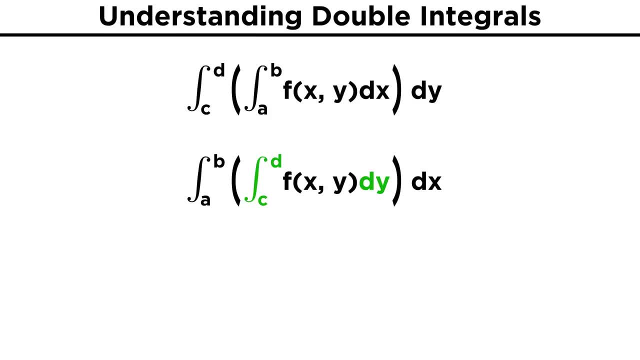 If we wanted to take the y-integral first, we would write it like this instead, with the dy first and the y-integral on the inside. As long as we keep proper track of the variables and their bounds, we can integrate in any. 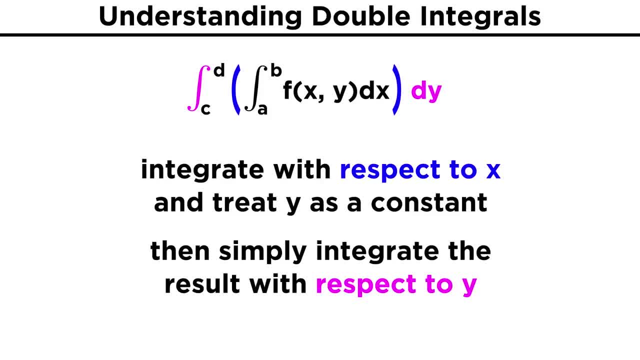 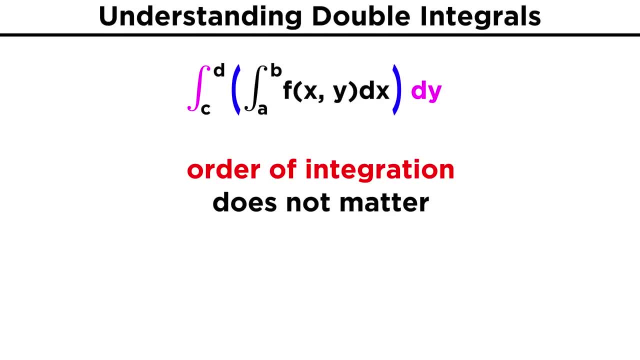 Then integrating the result over y, Just the same as we would for any variable. The order in which we do the integrations does not matter, as long as we keep track of which variable has which bounds. In this example, we see that dx is associated with the x integrand, which runs from A to. 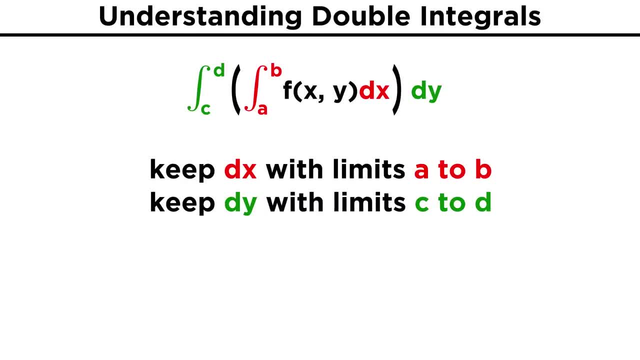 B, while dy is associated with the y integrand, which runs from C to D. If we wanted to take the y integral first, then we would have to do the same thing over x and then we would integral first. we would write it like this instead: with the dy first and the y integral. 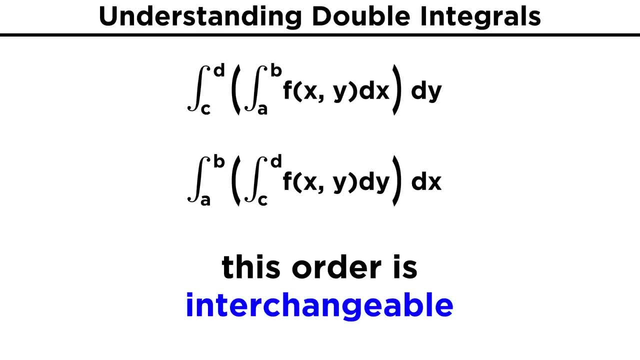 on the inside. As long as we keep proper track of the variables and their bounds, we can integrate in any order we want In more complex problems. this freedom lets us choose the order which will give the boundaries that are the simplest to express. 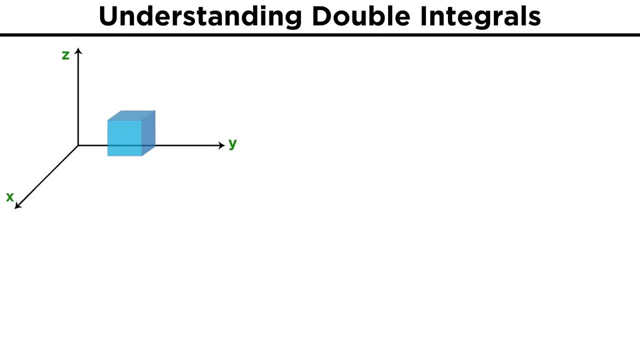 When we are looking for a volume within a rectangular region in the xy plane, double integrals are extremely straightforward. For example, let's try to find the volume under the function: f equals one plus four, xy, where x ranges from zero to one and y ranges from one to three. 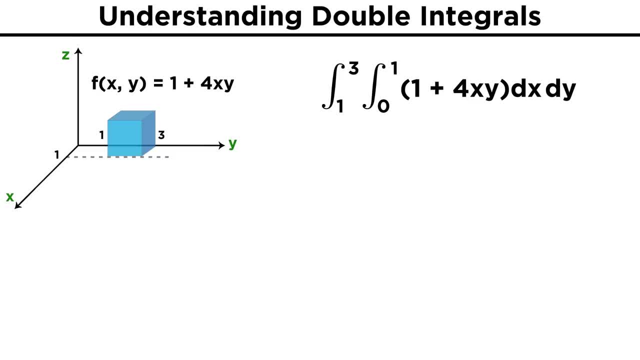 The volume will be given by the double integral. here, Let's go ahead and integrate over x first. Integrating over x, we will treat y as a constant and find the antiderivative with respect to x, which will be x plus two x squared y, which we will then evaluate from zero to. 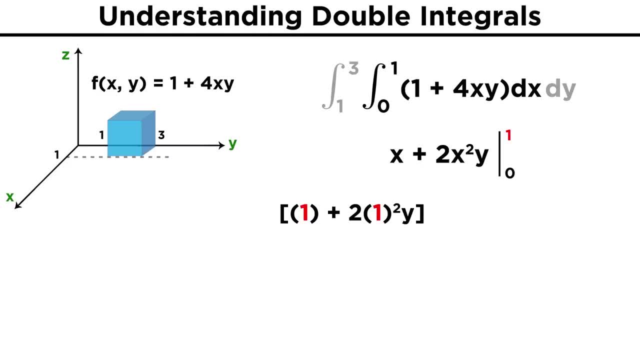 one. Plugging in x equals one. we get one plus two y, and then we must subtract the result when evaluated at x equals zero, which is just zero. So after evaluating the first integral, we are left with the integral of one plus two. 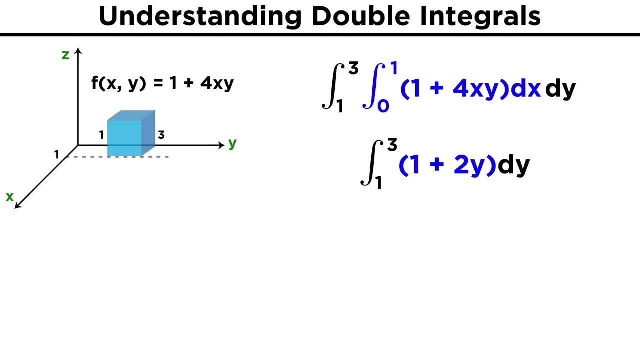 y with respect to y from one to three. We treat this the same as any integral over x. we just have a different variable to work with. The antiderivative with respect to y will be y plus y squared, which we will now evaluate. 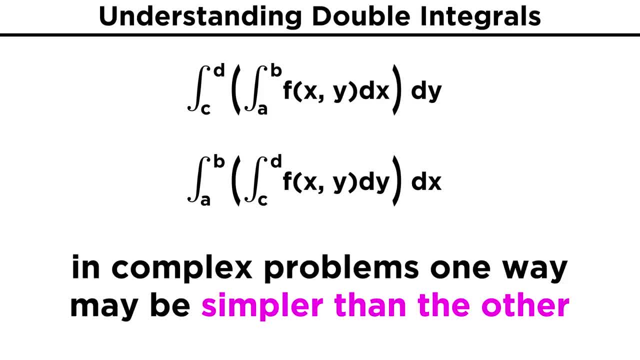 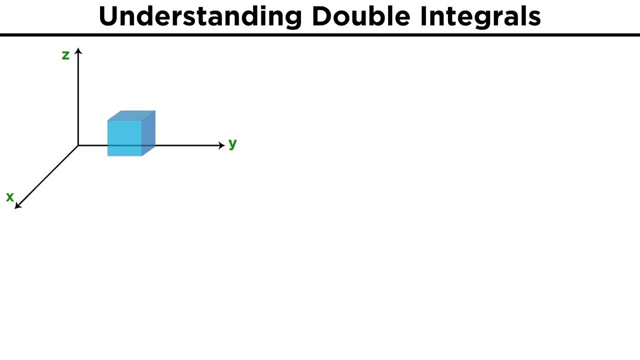 order we want In more complex problems. this freedom lets us choose the order which will give the boundaries that are the simplest to express When we are looking for a volume within a rectangular region in the x-y plane. we are looking for a volume within the x-y plane. 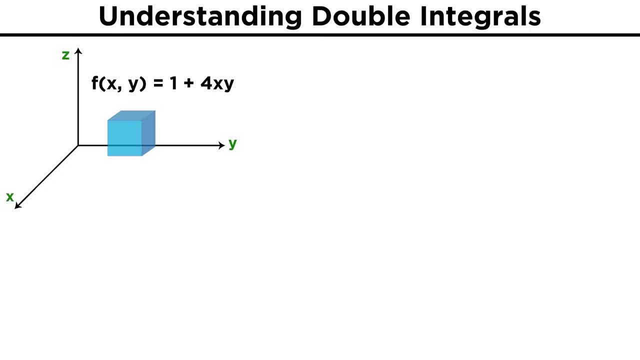 Double integrals are extremely straightforward. For example, let's try to find the volume under the function f of x comma. y equals one plus four, xy. where x ranges from zero to one and y ranges from one to three, The volume will be given by the double integral here. 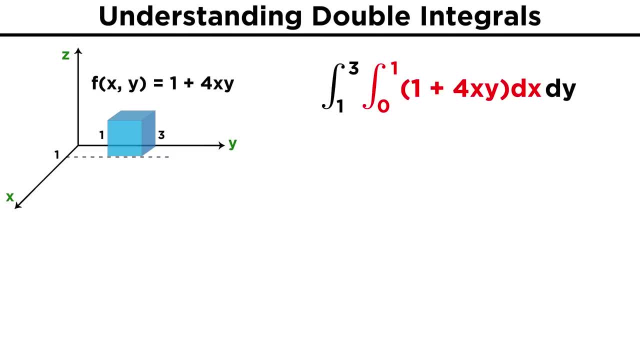 Let's go ahead and integrate over x first. Integrating over x, we will treat y as a constant. The volume will be the antiderivative with respect to x, which will be x plus two x squared y, which we will then evaluate from zero to one. 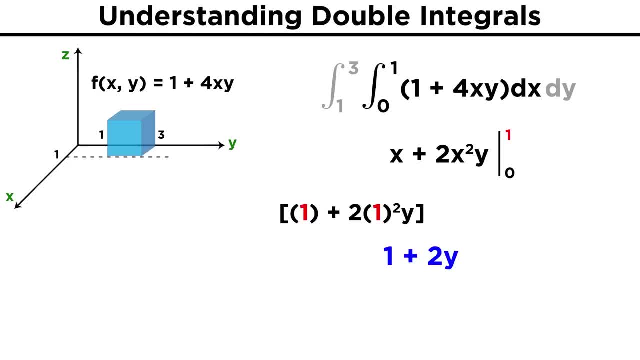 Plugging in x equals one, we get one plus two y, and then we must subtract the result when evaluated at x equals zero, which is just zero. So, after evaluating the first integral, we are left with the integral of one plus two y with respect to y, from one to three. 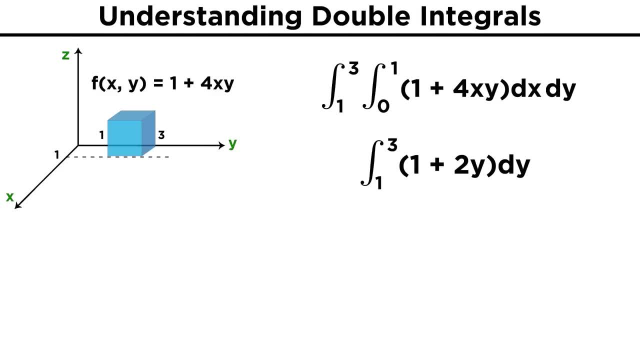 We treat this the same as any integral over x, we just have a different variable to work with. The antiderivative with respect to y will be y plus y squared, which we will now evaluate from one to three. Plugging in y equals three, we get three plus nine. then subtract the evaluation at y equals. 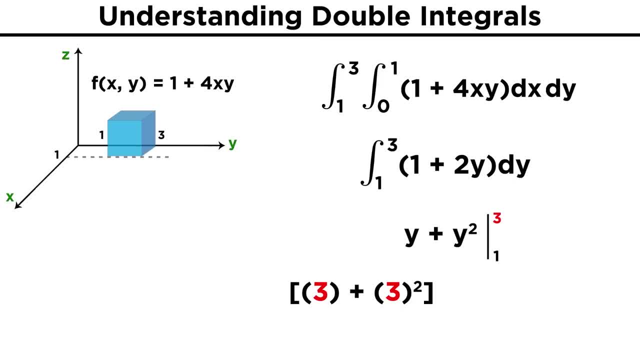 from one to three. Plugging in y equals three, we get three plus nine. Then subtract the evaluation at y equals one, which is one plus one, We get twelve minus two, which is ten. This is the result of our double integral and the volume of this section under the surface. 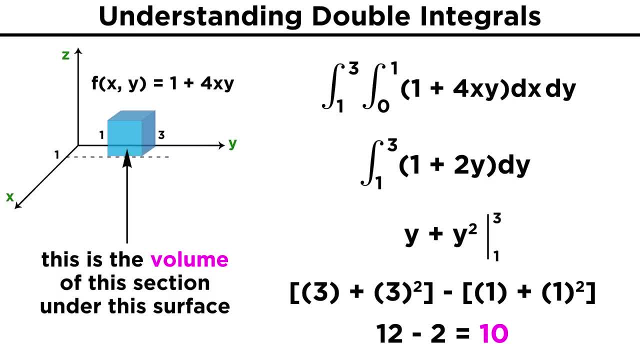 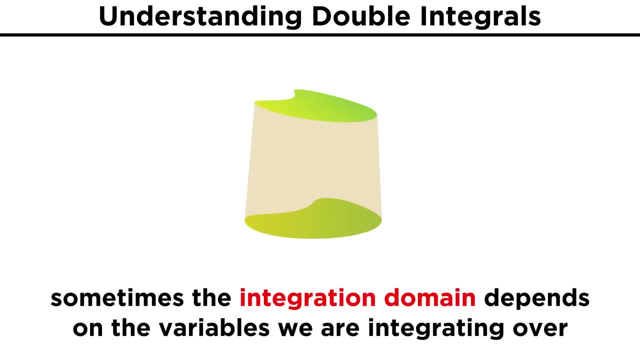 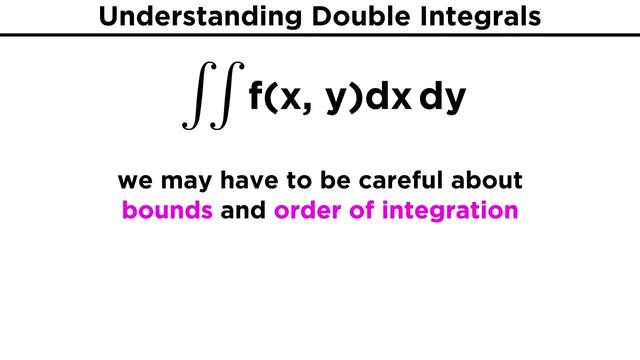 one plus four xy. What ends up making multiple integrals tricky is when the integration domain depends on the variables we're integrating over, For example, when the region we are considering in the xy plane involves curves rather than a rectangular area. In cases like this, we will have to be more conscious of how we write the bounds and the 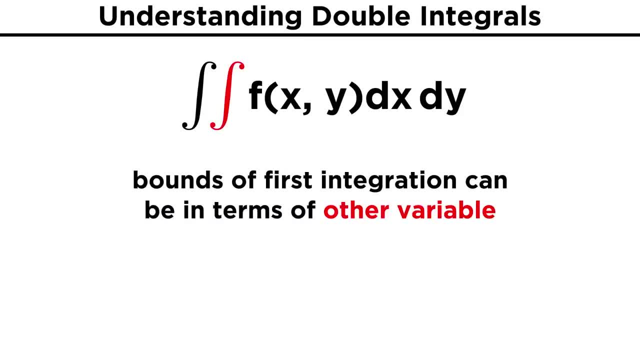 associated order of integration. What is likely to happen is that the bounds for the first integration will include the other variable, while the bounds for the second integration must be numbers to get a final result that is also a number. This is an important aspect to remember when thinking about the boundaries. 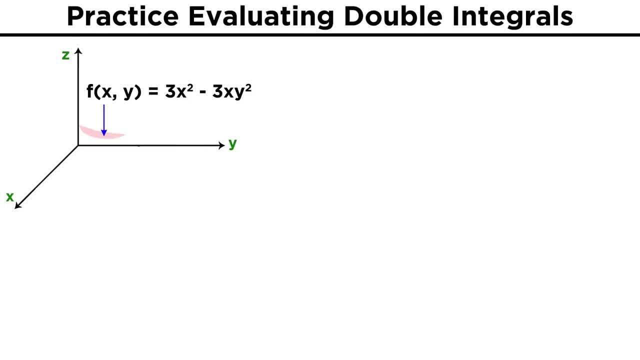 Thank you. Let's consider our surface to integrate to be given by the function f of x comma. y equals three x squared minus three xy squared, and we want to find the volume in this shaded region between y equals x squared and y equals two x. 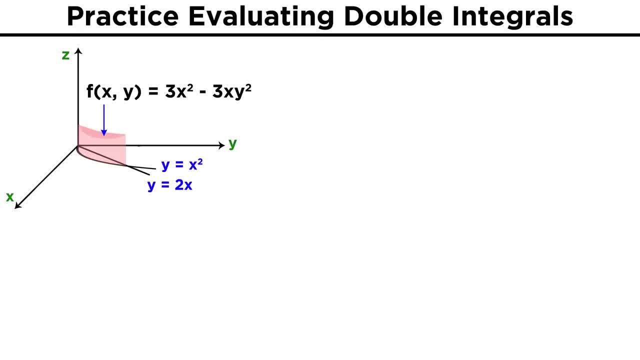 It's here that the challenge of establishing our boundaries from this information starts to present itself. There are two ways to go about this problem, but first we must take a look at the functions that determine our bounds, Because we have curves where x and y are related to each other. as our boundary, we must take 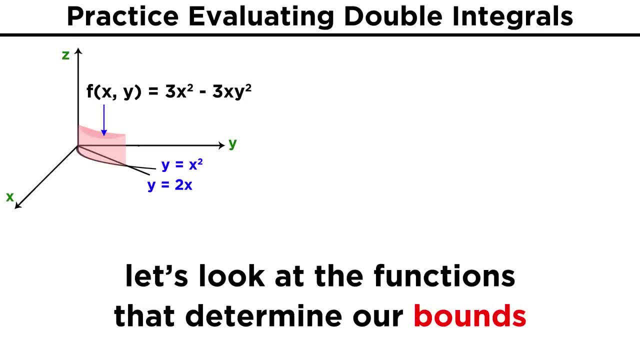 that relation into account in our integration. First we must establish where exactly our boundary begins and ends. We know we want this area between the functions y equals two x and y equals x squared. but we must determine the start and end points ourselves. 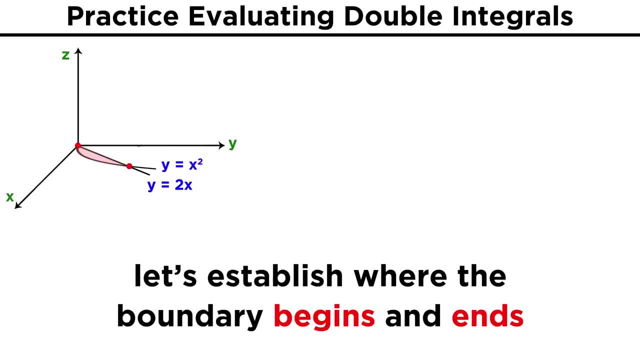 In this case, y equals two x and y equals x squared. In this case, y equals two x and y equals x squared. They will be the points where the functions intersect or where two x equals x squared. By simply moving two x to the other side, we see this is the same as zero equals x squared. 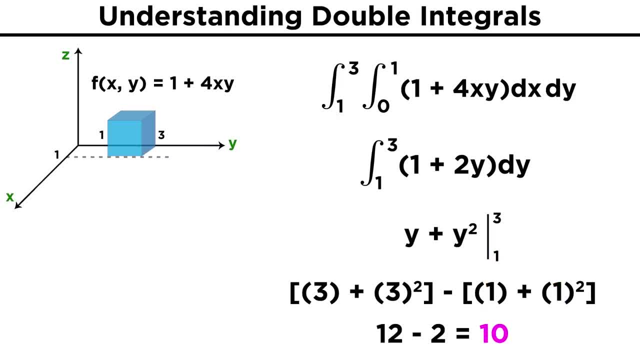 one, which is one plus one, We get twelve minus two, which is ten. This is the result of our double integral. We are left with the antiderivative with respect to y, which is one plus one. This is the result of our double integral and the volume of this section under the surface. 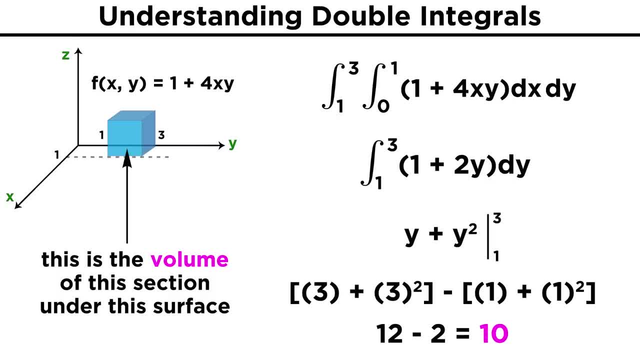 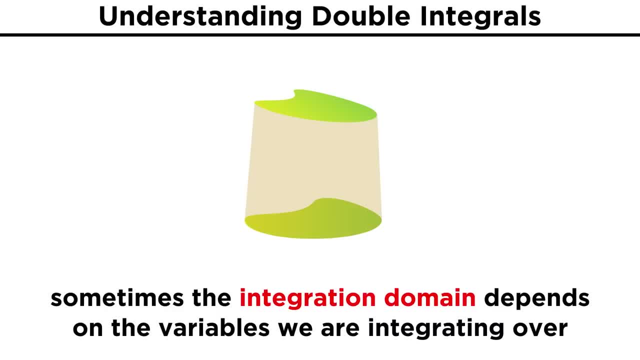 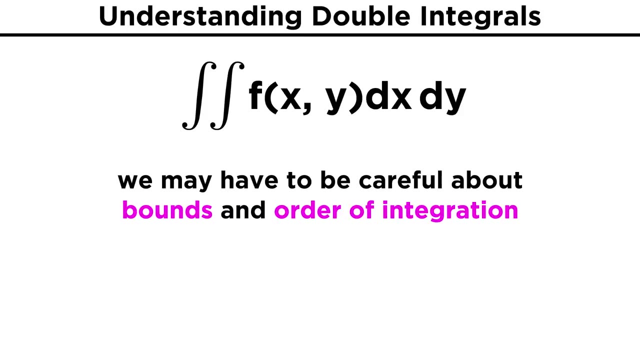 one plus four xy. What ends up making multiple integrals tricky is when the integration domain depends on the variables we're integrating over, For example, when the region we are considering in the xy plane involves curves rather than a rectangular area. In cases like this, we will have to be more conscious of how we write the bounds and 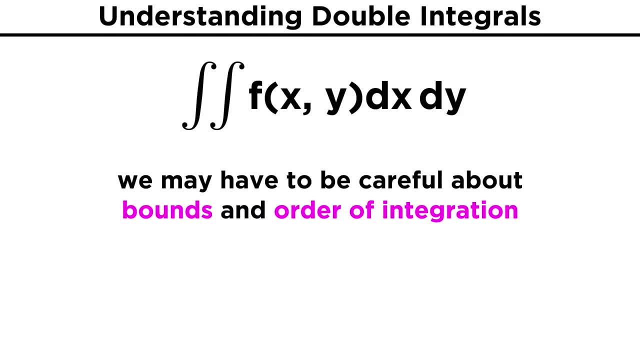 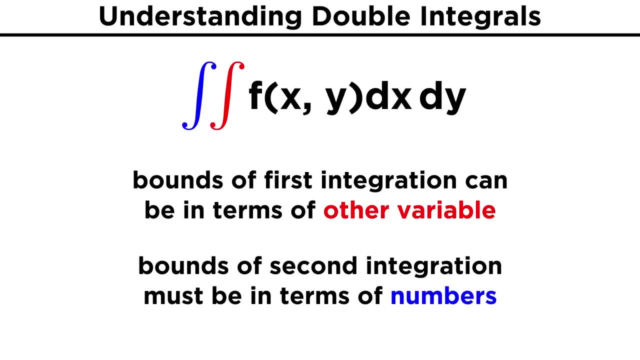 the associated order of integration. What is likely to happen is that the bounds for the first integration will include the other variable, while the bounds for the second integration must be numbers to get a final result that is also a number. This is an important aspect to remember when thinking about the boundaries. 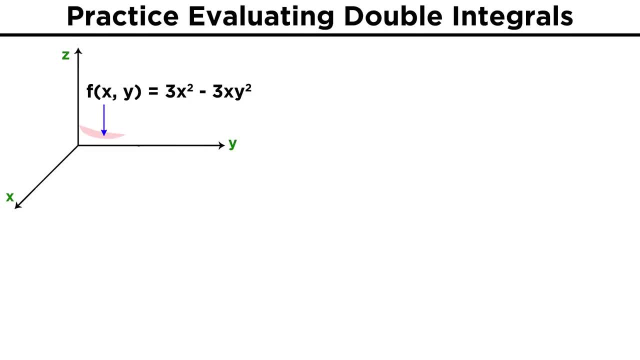 Let's consider our surface to integrate, to be given by the function integration f of x comma. y equals three x squared minus three xy squared, and we want to find the volume in this shaded region between y equals x squared and y equals two x. 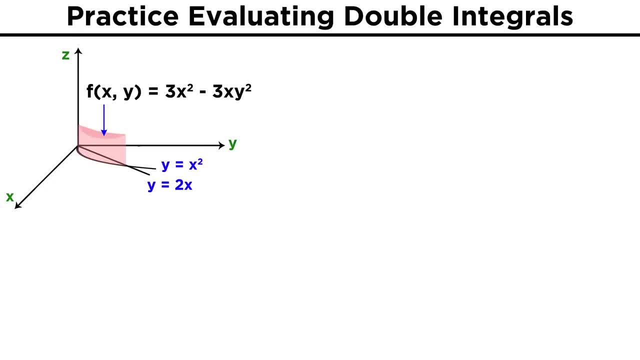 It's here that the challenge of establishing our boundaries from this information starts to present itself. There are two ways to go about this problem, but first we must take a look at the functions that determine our bounds, Because we have curves where x and y are related to each other. 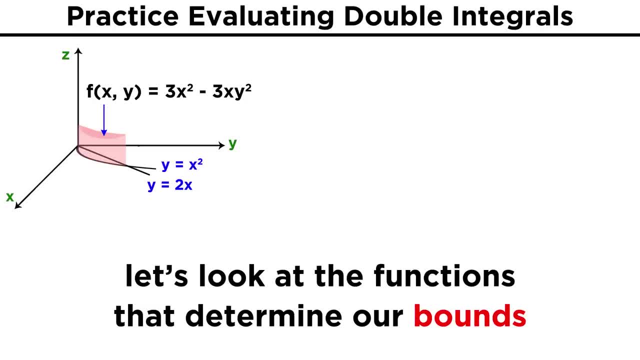 As our boundary. we must take that relation into account in our integration. First we must establish where exactly our boundary begins and ends. We know we want this area between the functions y equals two x and y equals x squared. but we must determine the start and end points ourselves. 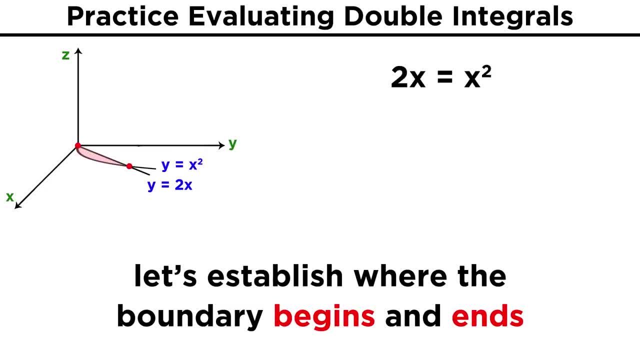 In this case, they will be the points where the functions intersect or where two x equals x squared. By simply moving two x to the other side, we see this is the same as zero equals x squared minus two x which, factored, gives x times x minus two. 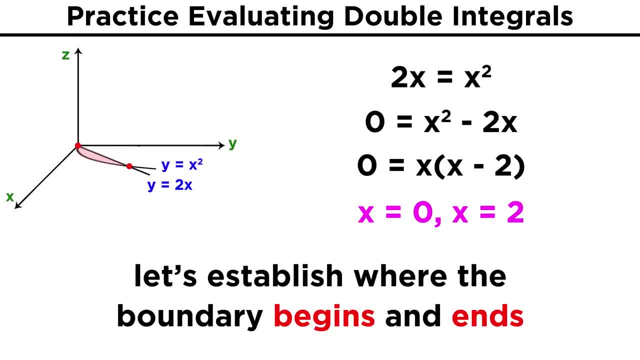 This means that our two points of intersection are x equals zero and x equals two. We can then get the y coordinates of the two points by plugging these values into either curve: Plugging in x equals zero, into y equals two. x gives y equals zero. 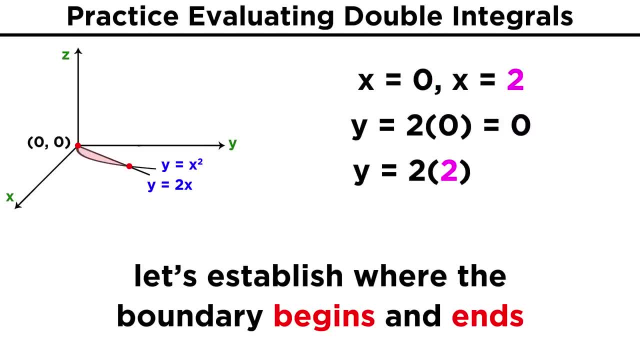 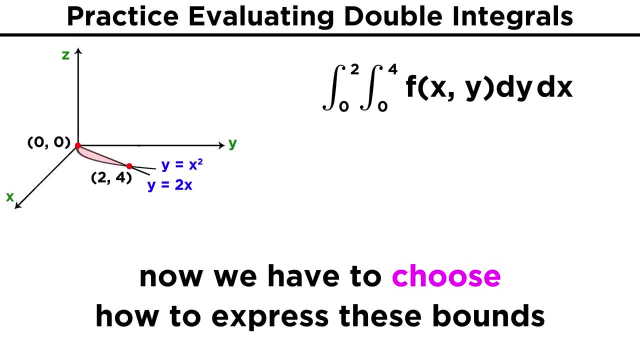 So our first coordinate is zero, zero. Plugging in x equals two into y equals two, x gives y equals four. so our second coordinate is two, four. Now is the point where we must choose how to express these bounds. We just found the points of interest on the x and y axis. 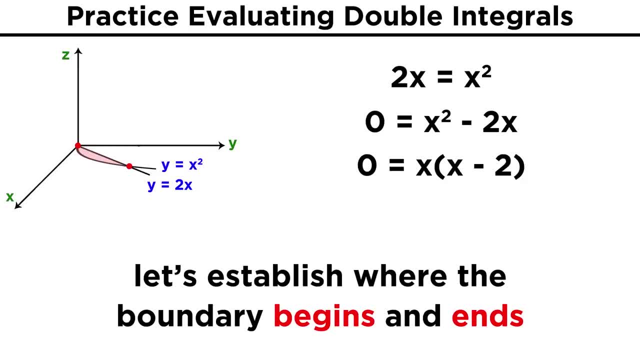 minus two. x which factored, gives x times x minus two. This means that our two points of intersection are x equals zero and x equals two. We can then get the y coordinates of the two points by plugging these values into either curve. 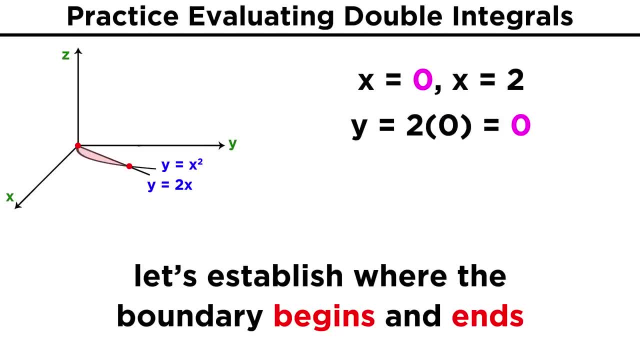 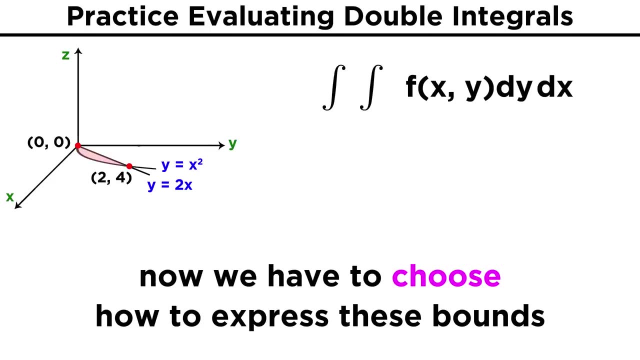 Plugging in x equals zero into y equals two. x gives y equals zero. so our first coordinate is: Plugging in x equals two into y equals two. x gives y equals four. so our second coordinate is: Now is the point where we must choose how to express these bounds. 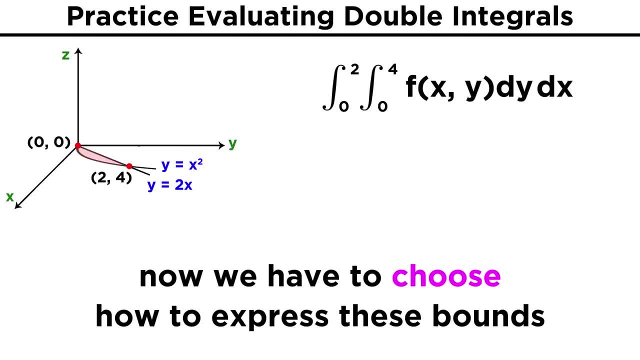 We just found the points of interest on the x and y axis. Our x coordinate can run from zero to two And our y coordinate can run from zero to four. However, using both these bounds gives us the rectangular area here, not the area between. 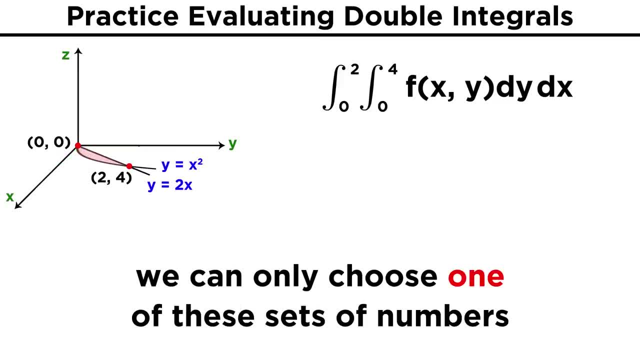 the curves. Instead of using both, we must choose one, and then the curves will become the bounds for the other variable. If we choose to run x from zero to two, then y must run from the lower curve to the higher curve, in this case from x squared to two x. 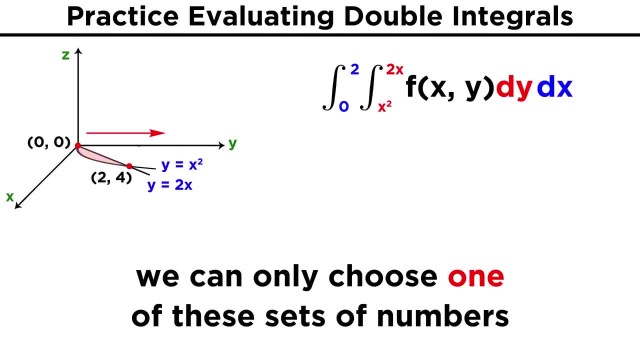 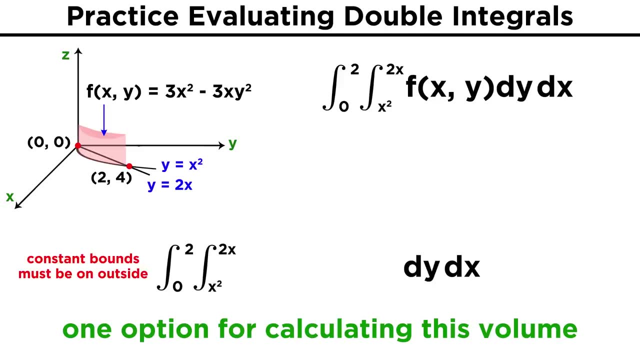 We always must choose the lower values as our lower bounds and the higher values as our upper bounds, otherwise we will be making an error in sign. So for our volume calculation we have the integration over x, from zero to two, the integration over y, from x squared to two, x of three, x squared minus three, x y squared, dy, dx. 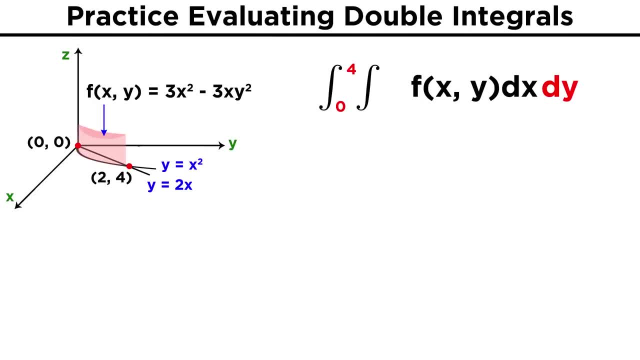 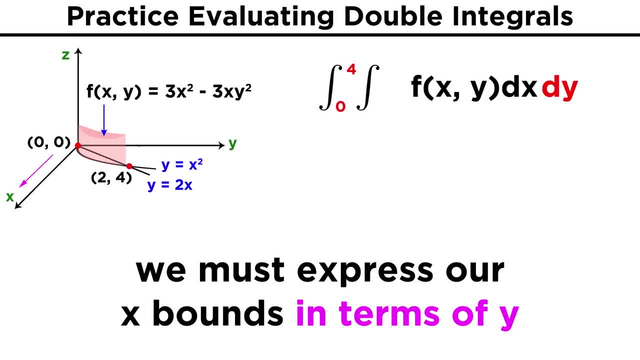 In this case we must now make our x bounds run from the lowest or leftmost curve. We are now wanting to start x at its lowest value relative to the curves going to higher values. so y equals two. x is now our lower bound for x and y equals x. squared will be. 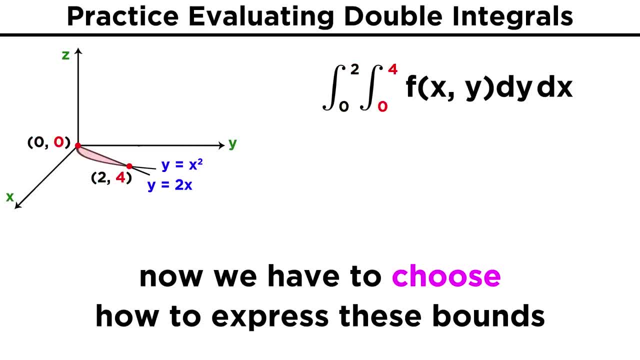 Our x coordinate can run from zero to two and our y coordinate can run from zero to four. However, using both these bounds gives us the y coordinate. Using both these bounds gives us the rectangular area here, not the area between the curves. 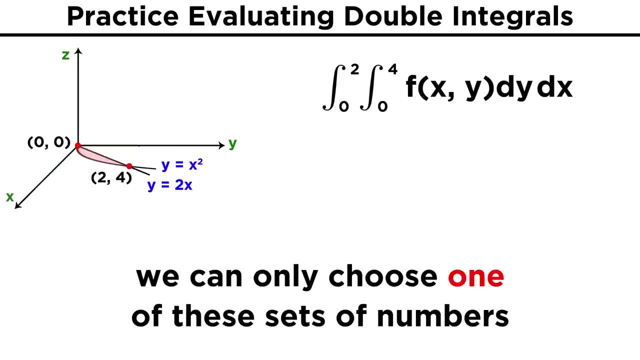 Instead of using both, we must choose one, and then the curves will become the bounds for the other variable. If we choose to run x from zero to two, then y must run from the lower curve to the higher curve, in this case from x squared to two x. 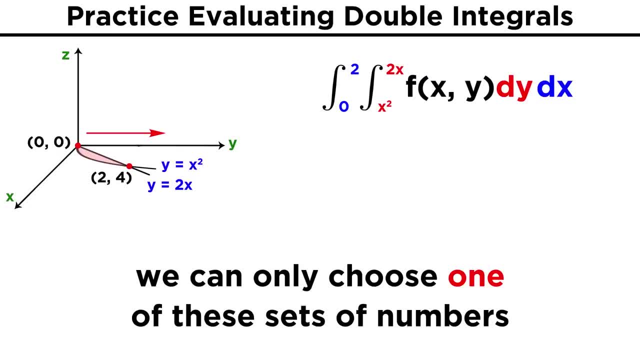 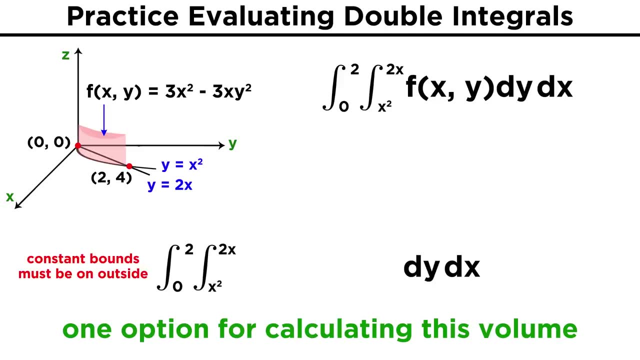 We always must choose the lower values as our lower bounds and the higher values as our upper bounds, otherwise we will be making an error in sign. So for our volume calculation we have the integration over x, from zero to two, the integration over y, from x squared to two, x of three, x squared minus three, x y squared, dy, dx. 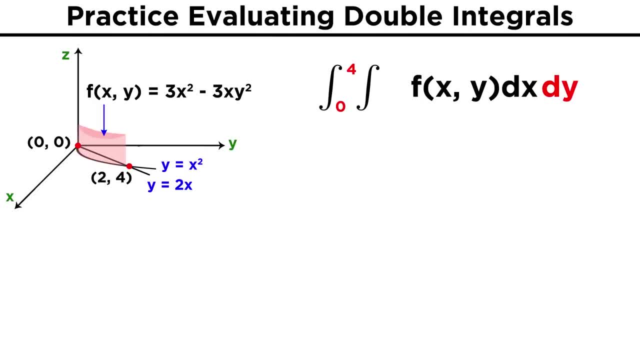 Let's step back and imagine we had chosen to let y run from zero to four instead. In this case, we must not choose the lower bounds, but instead choose the upper bounds as our upper bounds, otherwise we will be making an error in sign. 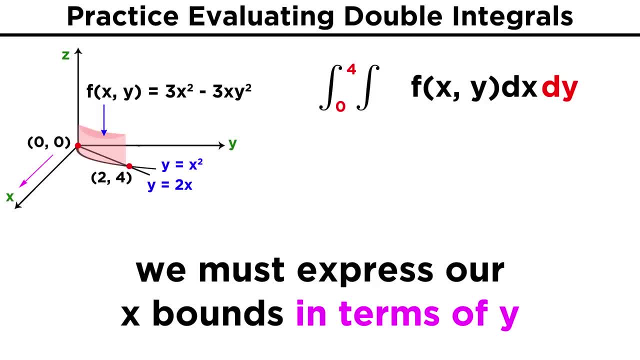 Let's now make our x bounds run from the lowest or leftmost curve. We are now wanting to start x at its lowest value relative to the curves going to higher values. so y equals two. x is now our lower bound for x and y equals x. squared will be. 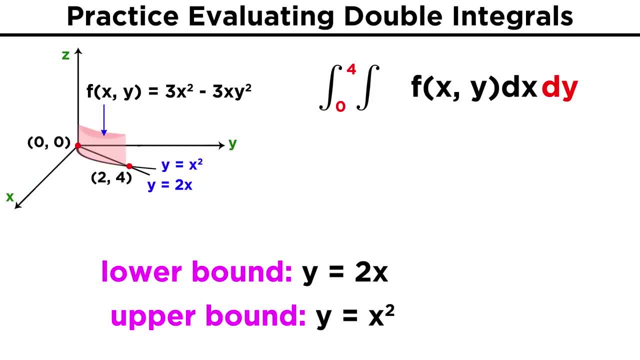 our upper bound. But there's a slight complication here. We want values of x to be our bounds for x, but these curves are expressed as values of y. For each curve we must express them in the form of: x equals some function of y. 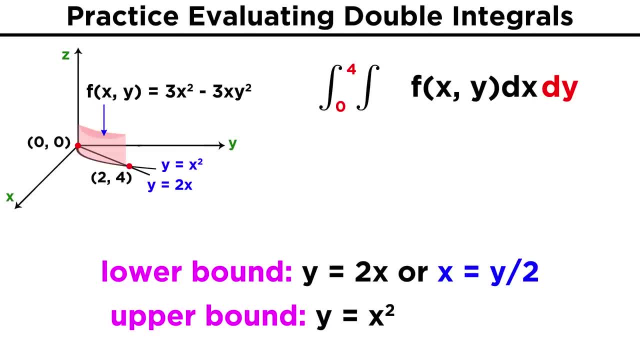 Both of these are relatively simple. For y equals two x. by dividing by two, we get x equals y over two. For y equals x. squared, we get x equals root y, Keeping track of which curve was the lower and upper bound. we want x to run from y over. 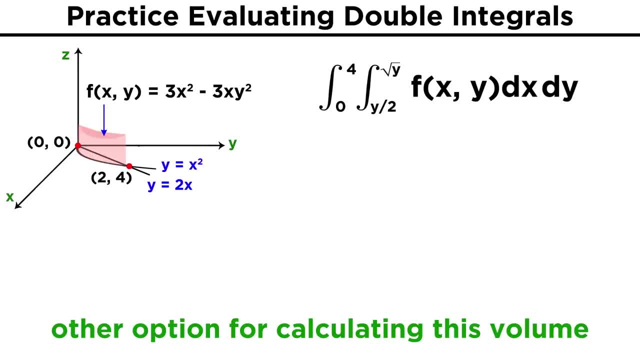 two to root y, So expressing our volume with these bounds, we end up with this. We end up with the integral over y, from zero to four, and integral over x, from y over two to root y. three, x squared minus three x, y squared, dx dy. 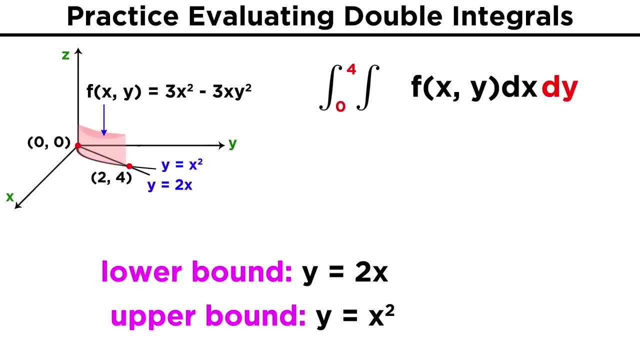 our upper bound. But there's a slight complication here. We want values of x to be our bounds for x, but these curves are expressed as values of y. so for each curve we must express them in the form of x equals some function of y. 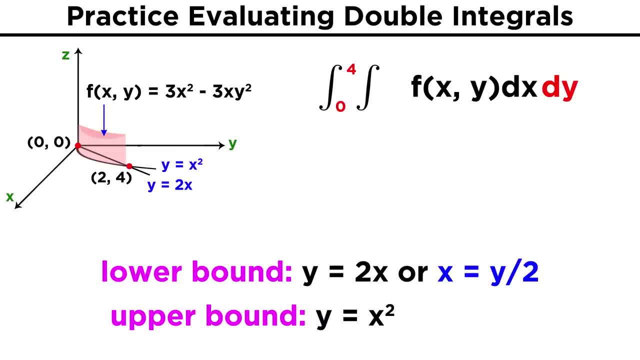 Both of these are relatively simple. For y equals two x. by dividing by two, we get x equals y over two. For y equals x. squared, we get x equals root y, Keeping track of which curve was the lower and upper bound. we want x to run from y over. 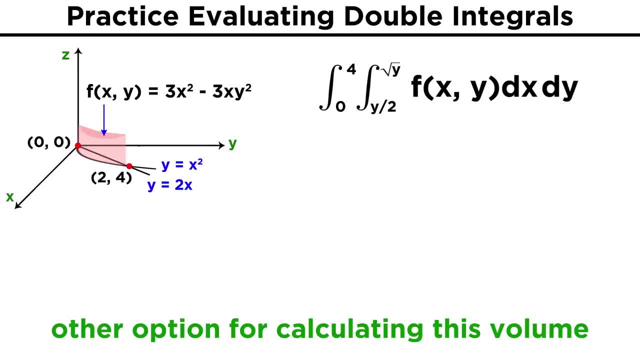 two to root y. So, expressing our volume with these bounds, we end up with the integral over y, from zero to four, and integral over x from y over two to root y. three x squared minus three x y squared. d x, d y. 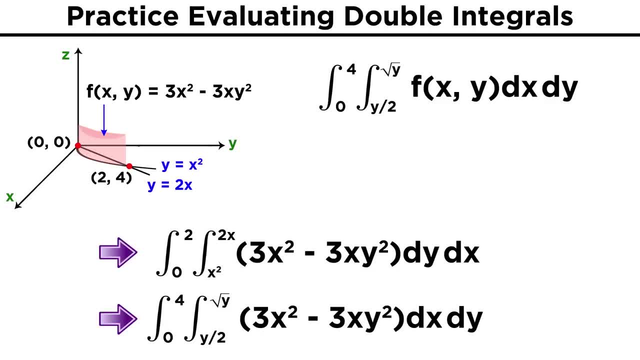 We now see that there are two ways to express this same volume: calculation. When establishing bounds, it's important to remember to keep the last bound equal to one running between two set values, after which we must express the other integral in terms of the curves of our boundary. 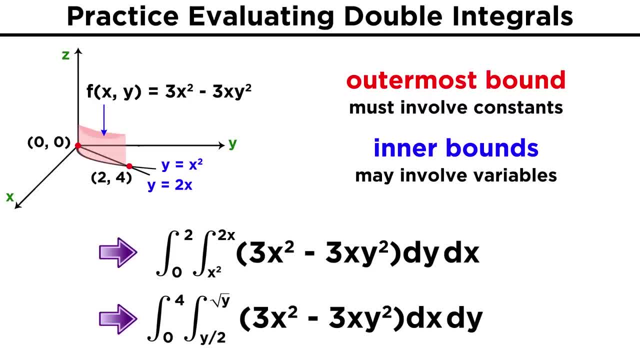 There are often times where one choice of bounds is more beneficial or makes things easier to calculate. For example, roots often complicate things as they are messier to deal with than whole integer exponents and can cause trouble dealing with negative values. 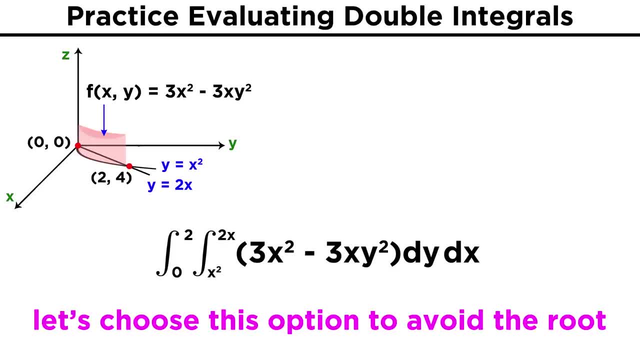 Now, let's actually go ahead and do a little bit of math. Let's go ahead and do a little bit of math. Let's do this integration To avoid the square root, we will choose to solve with the bounds where x runs from zero. 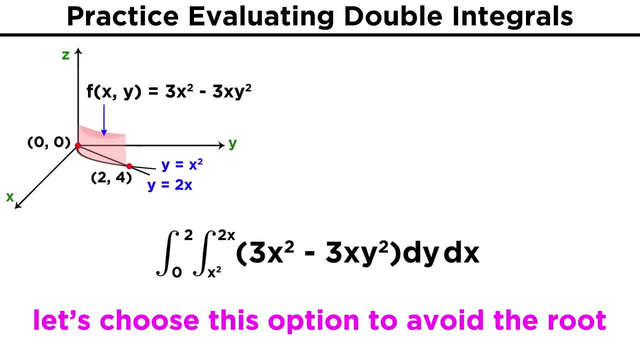 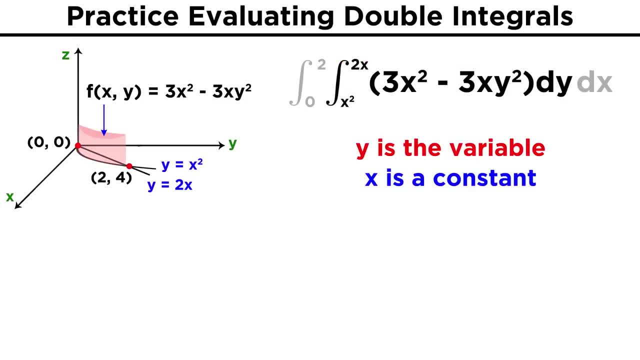 to two and y runs from x squared to two x. For this we must integrate with respect to y first, Taking the antiderivative with respect to y and treating x as a constant, we get three x squared y minus x, y cubed. 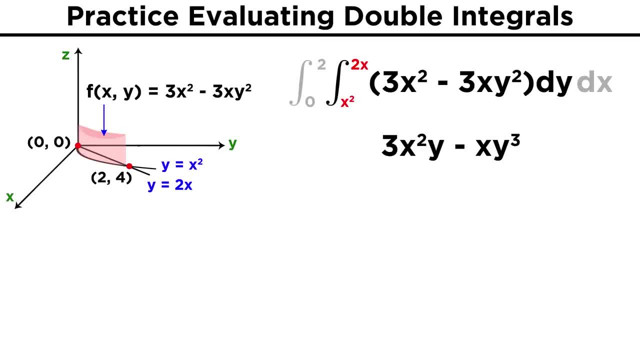 Now don't let the fact that our bounds involve x intimidate you. We still treat them as if they were numbers and evaluate our result from x squared to two x As such. we first plug in y equals two x into our antiderivative and get three x squared. 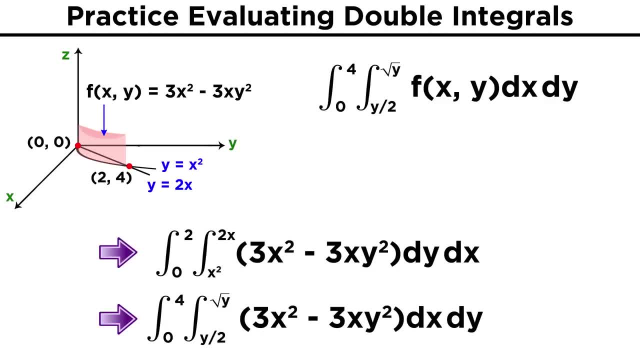 We now see that there are two ways to express this same volume calculation. When establishing bounds, it's important to remember to keep the last bound running between two set values, after which we must express the other integral in terms of the lower bound. So we're going to do that now. 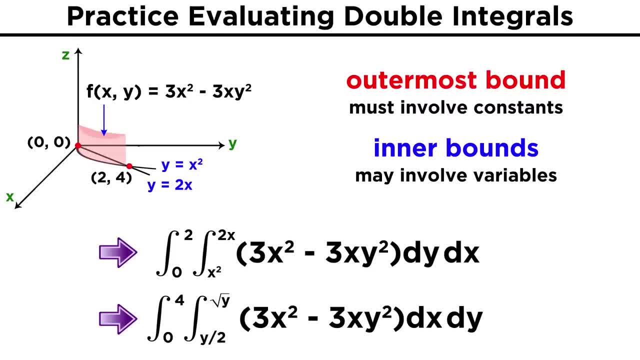 In terms of the curves of our boundary. There are often times where one choice of bounds is more beneficial or makes things easier to calculate. For example, roots often complicate things as they are messier to deal with than whole integer exponents and can cause trouble dealing with negative values. 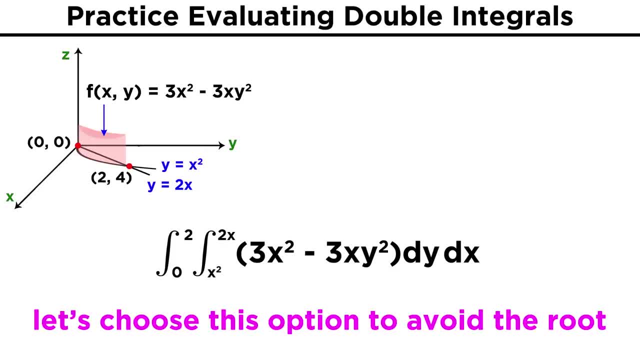 Now let's actually go ahead and do this integration. To avoid the square root, we will choose to solve with the bounds where x equals one over two. So we'll start with a bound where x runs from zero to two and y runs from x squared. 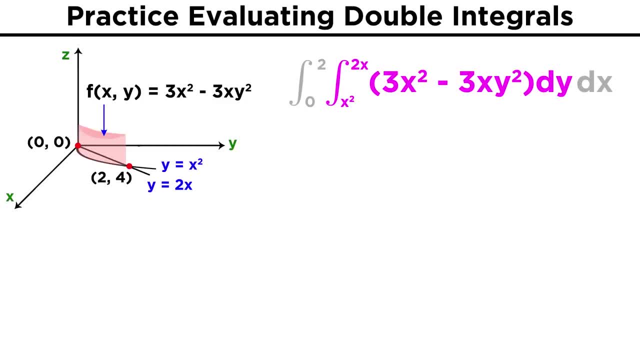 to two x. For this we must integrate with respect to y first, Taking the antiderivative with respect to y and treating x as a constant, we get three x squared, y minus xy cubed. Now don't let the fact that our bounds involve x intimidate you. we still treat them as if. 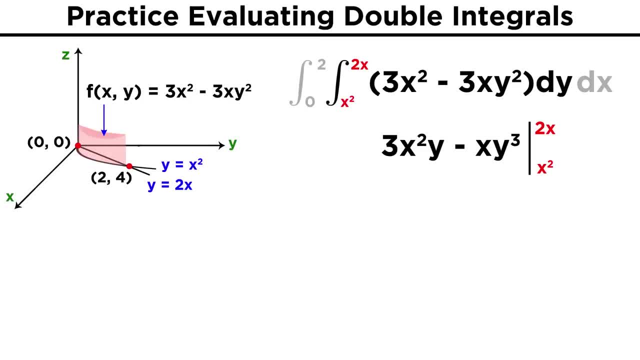 they were numbers and evaluate our result from x squared to two x As such. we first plug in y equals two x into our antiderivative and get three x squared times two x minus x times two x cubed. Then we subtract from that the other expression where we are plugging in y equals x squared. 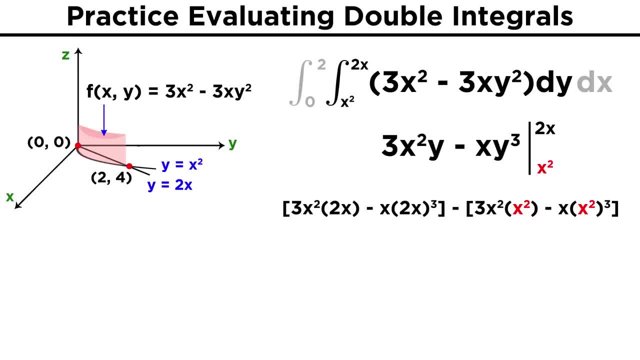 so we get minus three x squared times x squared minus x times x squared cubed. Simplifying from there, we are left with the integral over x of three x squared times x squared minus x times x squared cubed. So now we know x squared minus 6x cubed, minus 8x to the fourth, minus the quantity three. 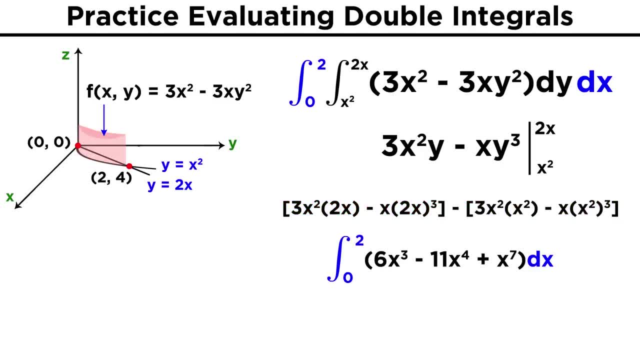 x to the fourth minus x to the seventh, or six x cubed minus eleven, x to the fourth plus x to the seventh, dx, where x runs from zero to two. We're now in the homestretch with just one last integral to evaluate. 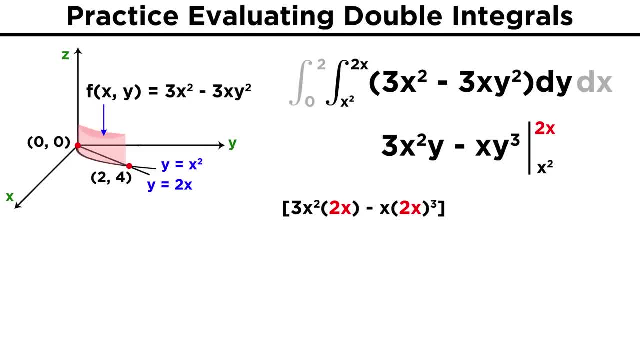 times two x minus x times two x cubed. Then we subtract from that the other expression where we are plugging in: y equals x squared, so we get minus three x squared times x squared minus x times two x squared minus x times. 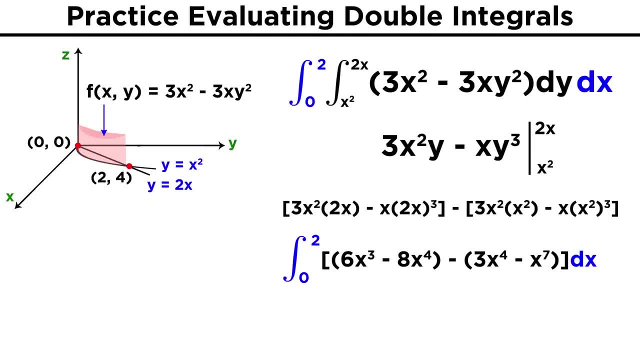 x squared cubed. Simplifying from there, we are left with the integral over x of six x cubed minus eight x to the fourth, minus the quantity three x to the fourth minus x to the seventh, or six x cubed minus eleven x to the fourth plus x to the seventh. dx where x runs from zero. 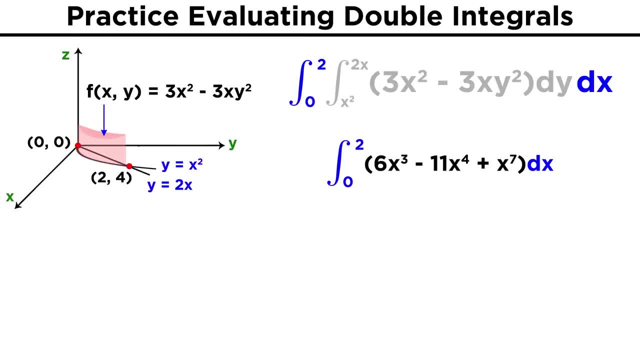 to two. We're now in the home stretch with just one last integral to evaluate. The antiderivative of y equals x squared minus x to the fourth, minus x to the seventh. dx, where x runs from zero to two, The integral of this expression becomes six x to the fourth over four minus eleven x. 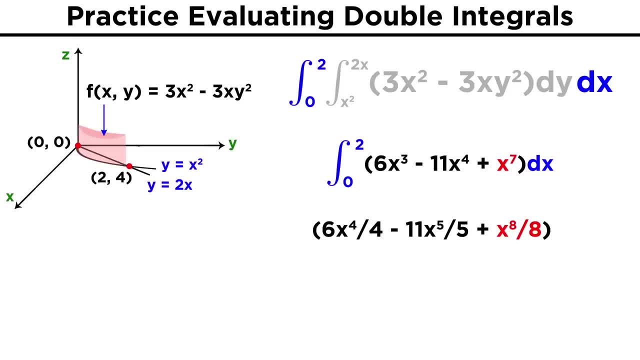 to the fifth over five, plus x to the eighth over eight. evaluated from zero to two, Plugging in two, we get six times two to the fourth over four minus eleven times two to the fifth over five, plus two to the eighth over eight. 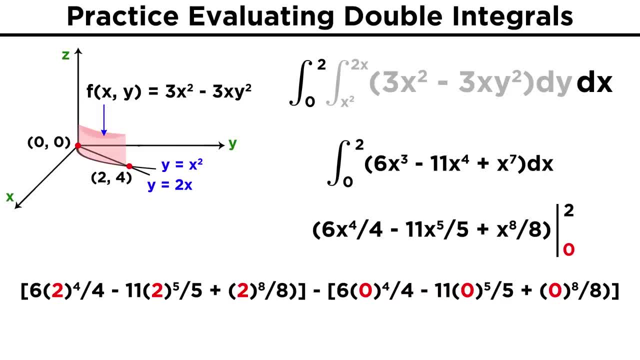 From this we must subtract the expression where we plug in: x equals zero, but this will simply be zero. We can then plug this into our antiderivative. We can then plug this into a calculator and find the volume to be negative fourteen point four or negative seventy-two fifths. 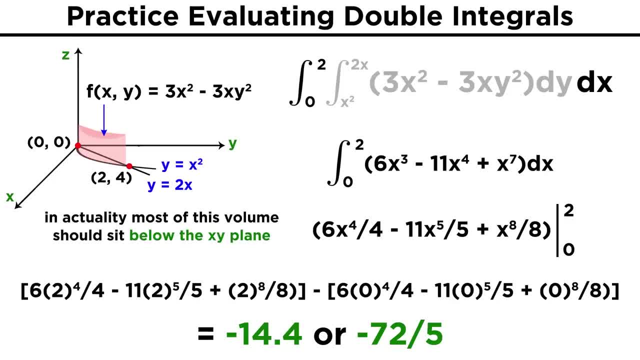 This negative value simply indicates that most of the surface- three x squared minus three xy squared- in this area is below the xy plane. And, to be clear, we would have gotten this same answer if we went through the calculation using the other way to express the bounds. we just decided that this way was easier. 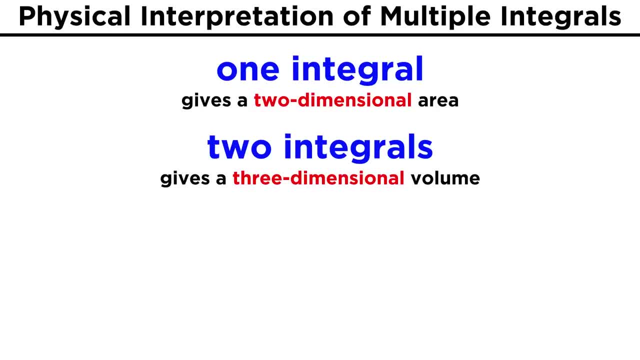 And we've solved this problem. As we can see, adding extra integrals is the same as adding extra dimensions, and our overall process does not change. Three integrals can be thought of as giving a hypervolume in four dimensions, Four integrals would give a hypervolume in five dimensions, and so on. 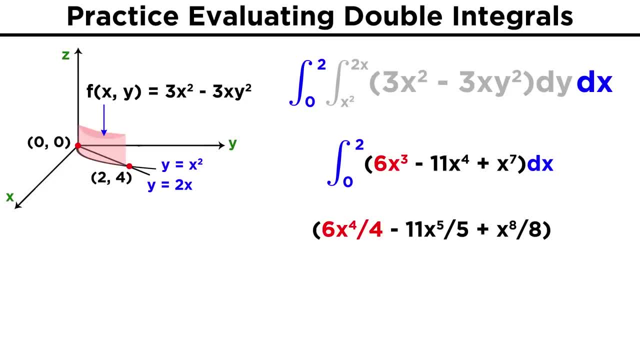 The antiderivative of this expression becomes six x to the fourth over four minus eleven x to the fifth over five plus six x cubed minus eight x to the fourth minus the quantity 5, plus x to the 8th over 8, evaluated from 0 to 2.. 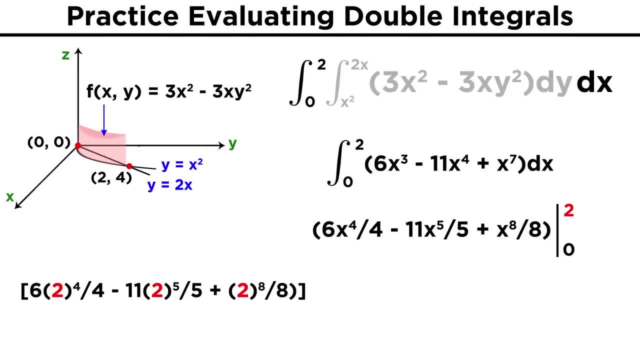 Plugging in 2, we get 6 times 2 to the 4th over 4,, minus 11 times 2 to the 5th over 5, plus 2 to the 8th over 8.. From this we must subtract the expression where we plug in: x equals 0, but this will. 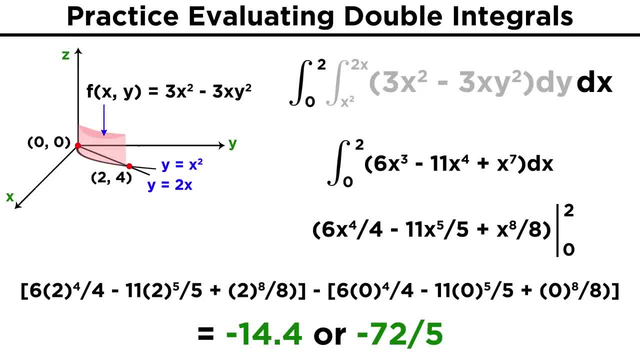 simply be 0. We can then plug this into a calculator and find the volume to be negative 14.4, or negative 72 fifths. This negative value simply indicates that most of the surface 3x squared minus 3xy squared. 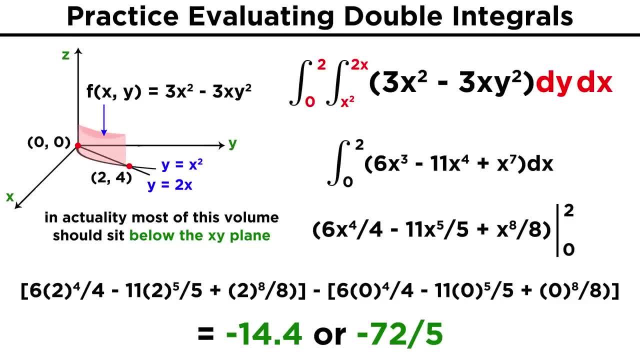 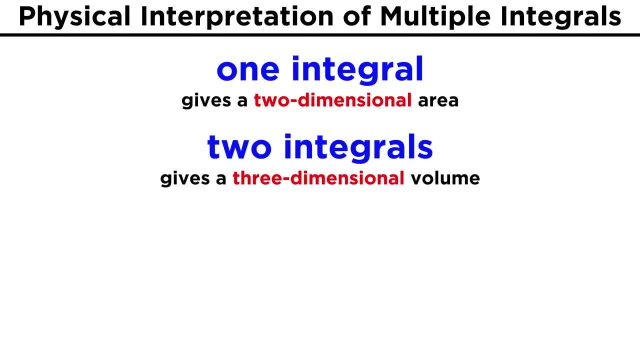 in this area is below the xy plane And, to be clear, we would have gotten this same answer if we went through the calculation using the other way to express the bounds. we just decided that this way was easier. As we can see, adding extra integrals is the same as adding extra dimensions, and our 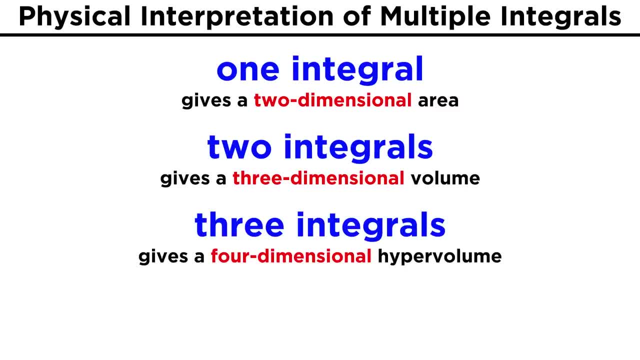 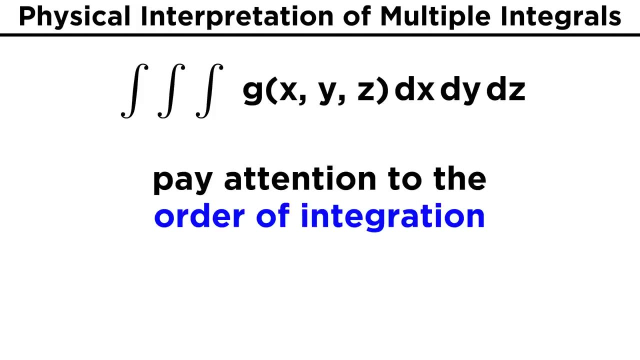 overall process does not change. Three integrals can be thought of as giving a hypervolume in four dimensions. Four integrals would give a hypervolume in five dimensions, and so on. Again, the most important thing to remember is the order of integration, and just take 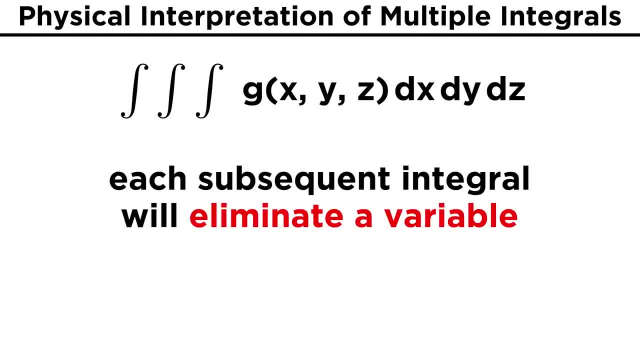 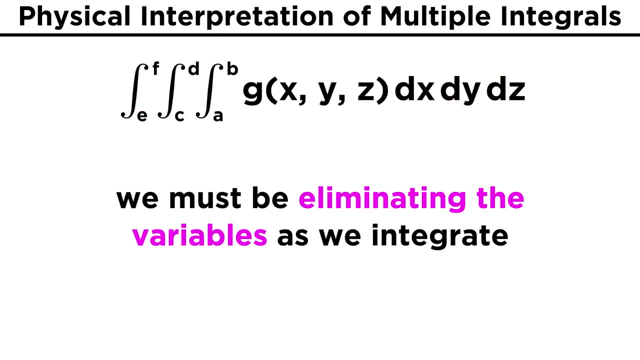 things one step at a time. A rule of thumb is to remember that each subsequent integral eliminates a variable. Thank you. For example, if we have a triple integral of g, where x runs from a to b, y runs from c to d and z runs from e to f, as we go through, each integral we must be eliminating. 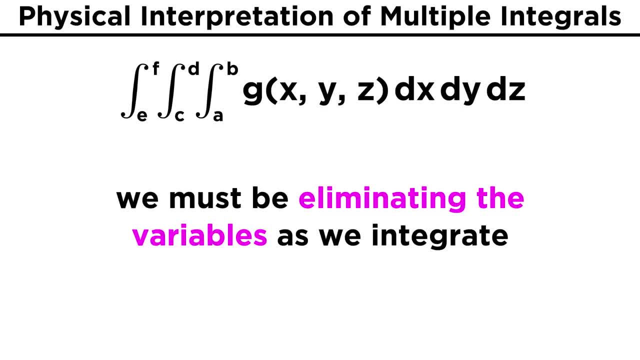 the variables x, y and z when we integrate each of them. Meanwhile, the bounds can still depend on other variables When setting them up, just keep in mind that the bounds are not always the same. Keep in mind the order and what possible variables can still go into the expression. 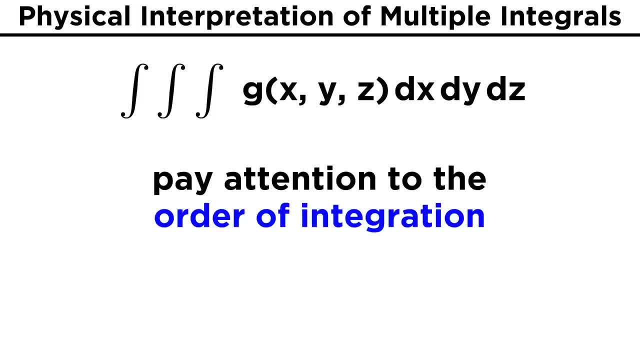 Again, the most important thing to remember is the order of integration and just take things one step at a time. A rule of thumb is to remember that each subsequent integral eliminates a variable. For example, if we have a triple integral of G where X runs. 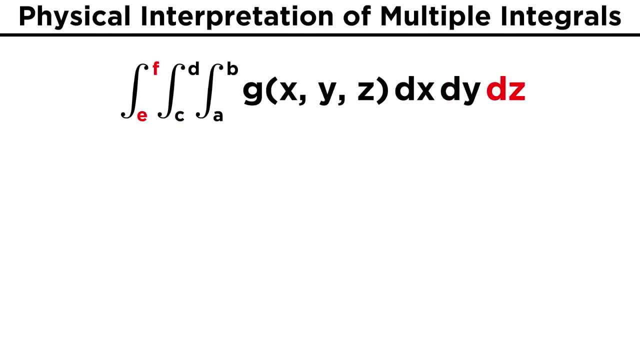 from A to B, Y runs from C to D and Z runs from E to F. as we go through each integral, we must be eliminating the variables X, Y and Z when we integrate each of them. Meanwhile, the bounds can still depend on other variables. 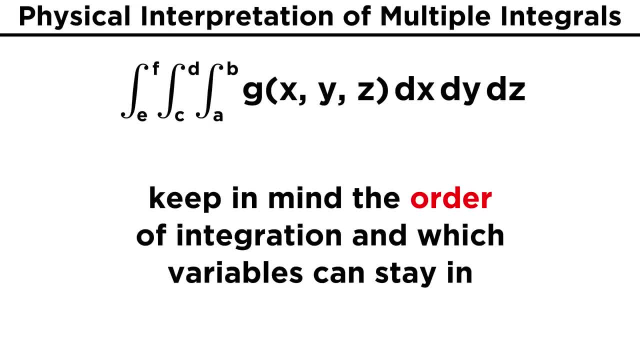 When setting them up, just keep in mind the order and what possible variables can still go into the expression without reintroducing ones that have already been integrated out. For this triple integral, if we integrate X first, its bounds A and B can depend on. 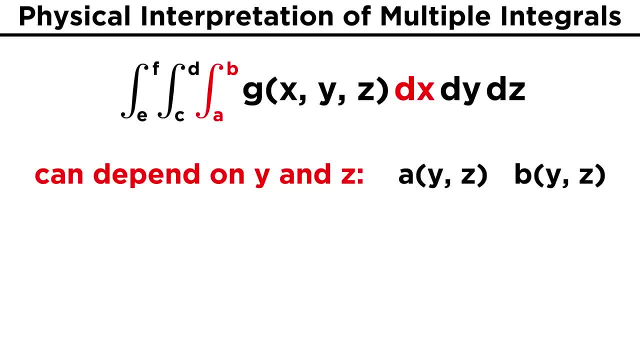 either of them Or of the other two variables, Y and Z. If we integrate Y, next the bounds C and D can no longer depend on X, but can still depend on Z. And finally, the last variable, Z, can only vary between two constants, as all the other. 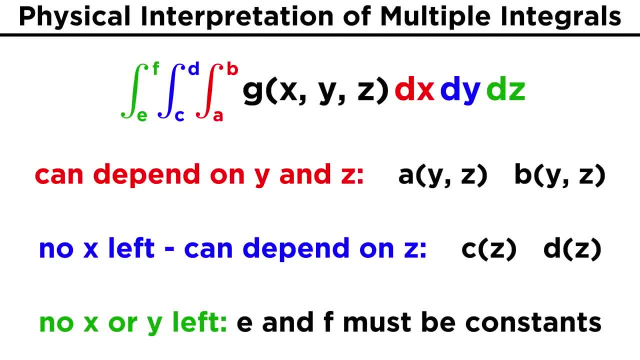 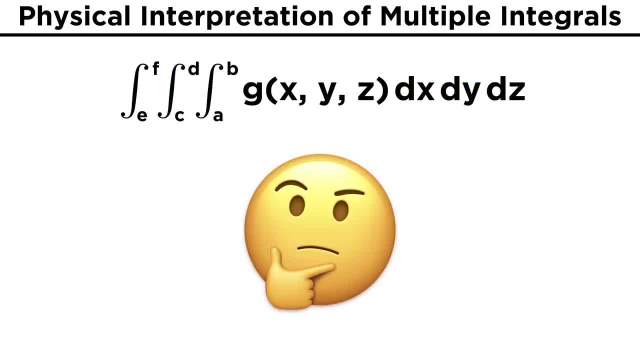 variables have been integrated out And of course, the bounds cannot have the same variable that is being integrated. There's an incredible depth to multiple integrations. There are multiple integrals that can't be covered in a single tutorial, but we've laid out the type of thinking needed to approach setting up bounds. 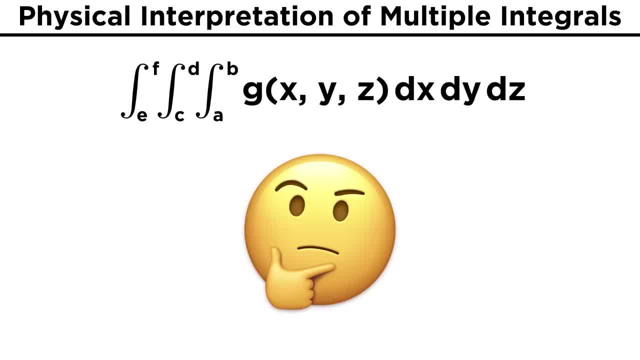 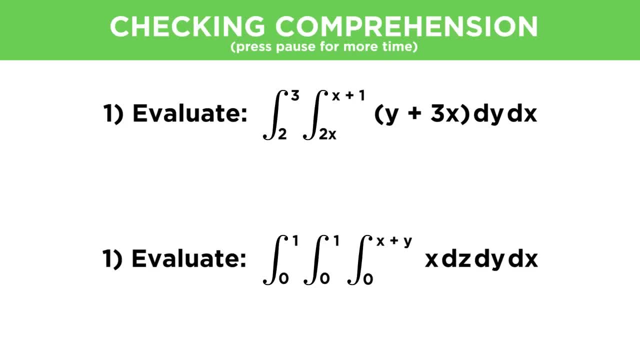 Multiple integrals are a key technique in a number of fields of math and science, so getting down the basics for these is key. With that covered, let's check comprehension. Thanks for watching, guys. subscribe to my channel for more tutorials. support me on. 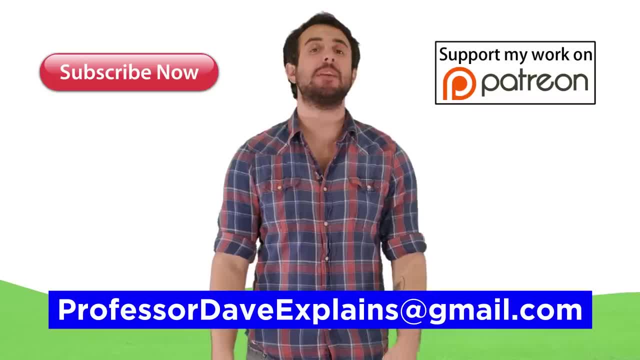 patreon, so I can keep making content. and, as always, feel free to email me, professordaveexplains at gmail dot com. I'll see you in the next video. Bye.